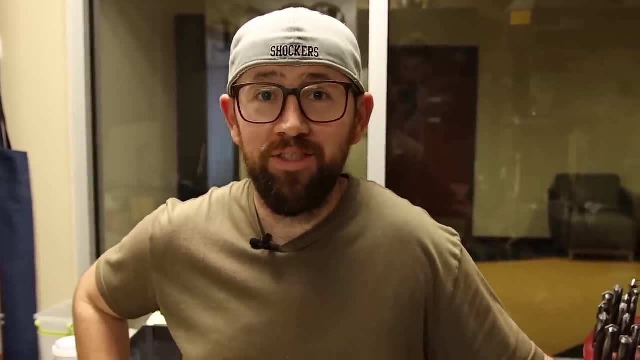 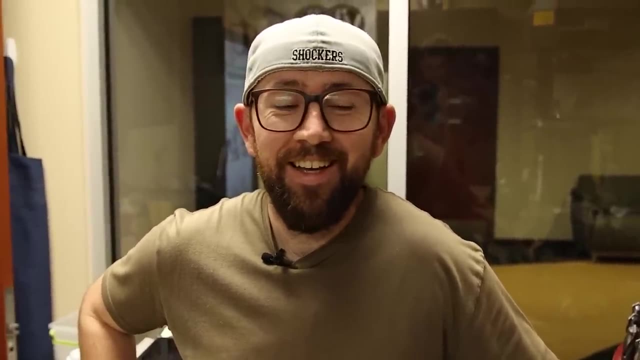 back over it- And you know, this was back in the day- when you can only have one ounce of side weight legally. We just discovered that this guy was blatantly cheating. He'd been using this ball in league tournaments and everything like that. So our first thought was: does this even? 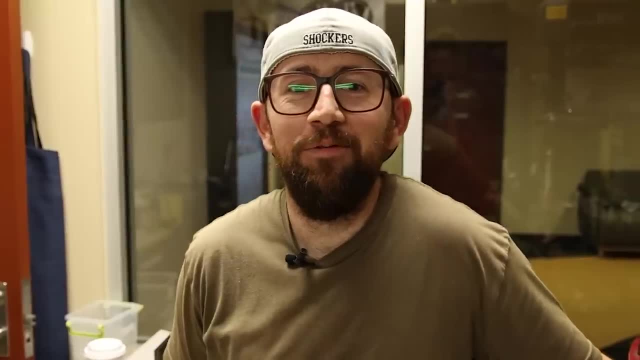 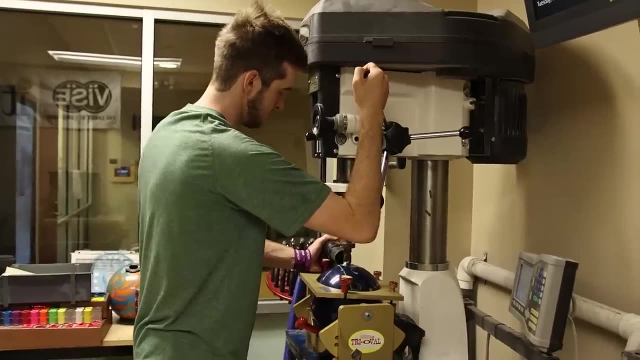 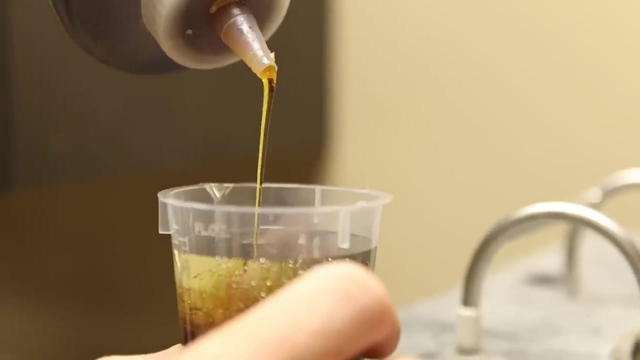 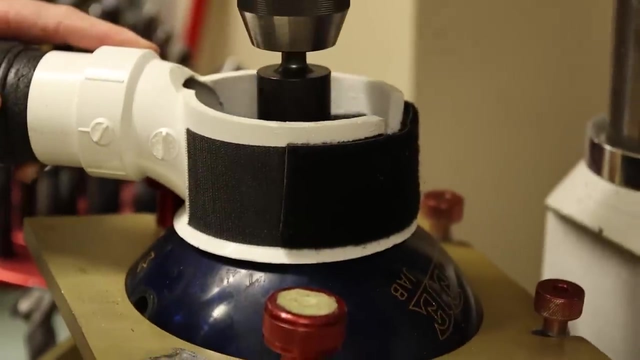 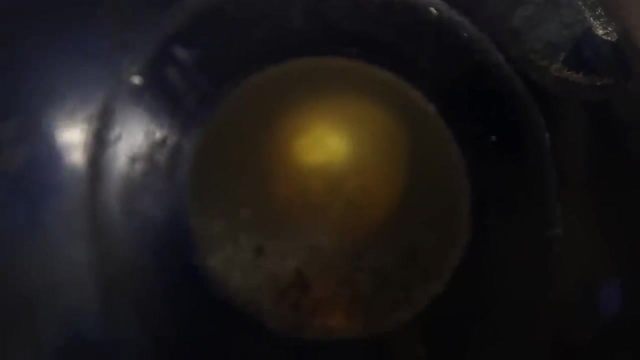 help. So Paki and I are going to run a little experiment today to see if adding a bolt to a ball actually does anything gooey background music illegal. We've done it with a regular plug. You'd really be able to see it, but time crunch, quick plug. 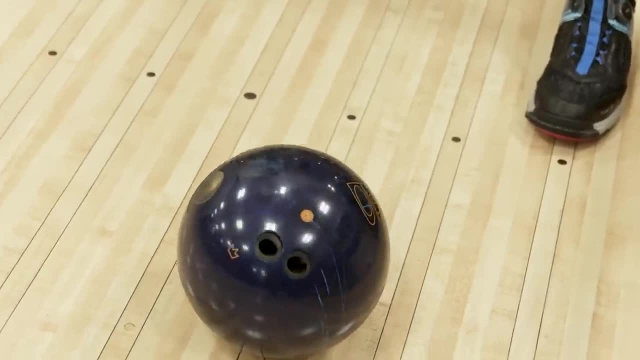 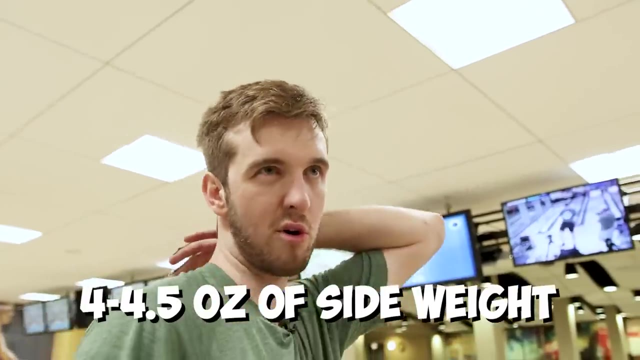 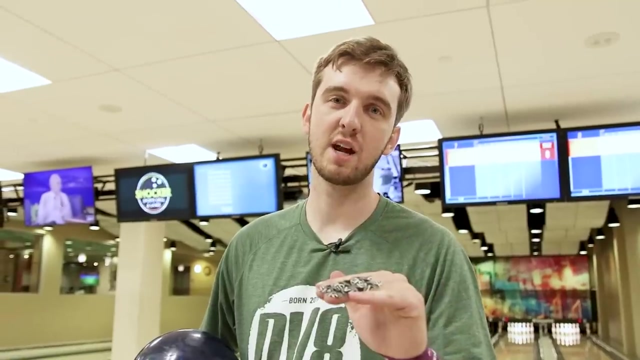 she's loping. she's really just a little side heavy. so estimating four to four and a half maybe, probably not five, but i mean over four for sure i'm gonna go straight into a game i'm not even gonna line up. i was playing like not 17, i was playing like 15 and it was hitting the pocket. 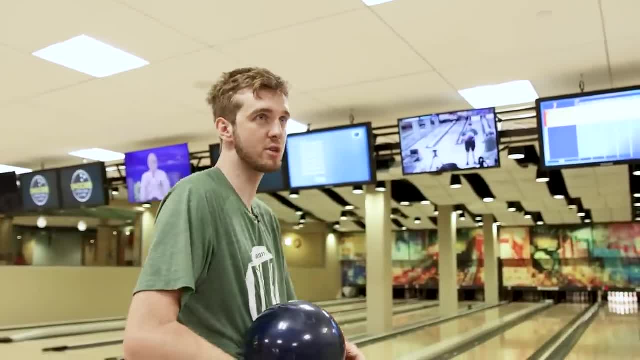 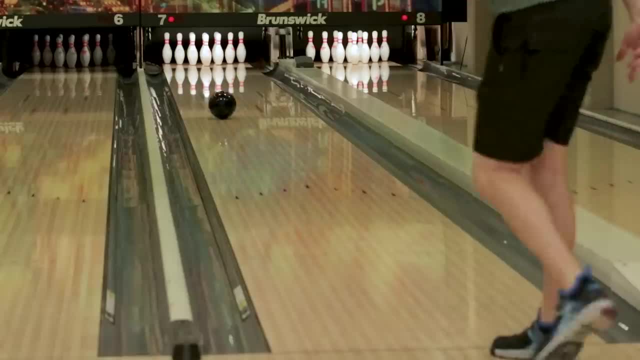 pretty good, so i don't know if this will help hurt. make a hook more. make a hook less. i tried to make a hook more of them. i'm gonna throw it from the same spot to start and we're just gonna go straight into the game. not a good shot. a little sticky from the- uh, the flying eagle. 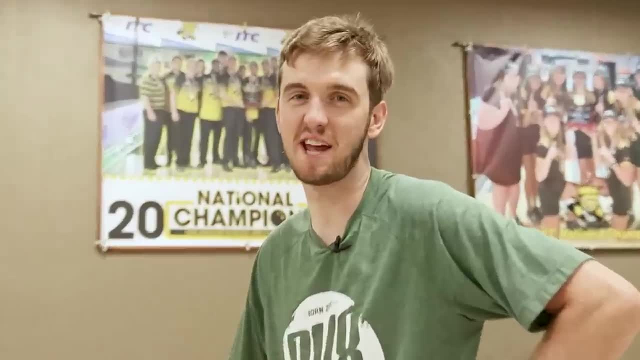 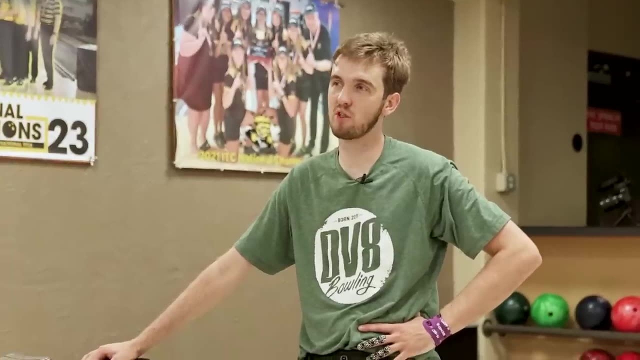 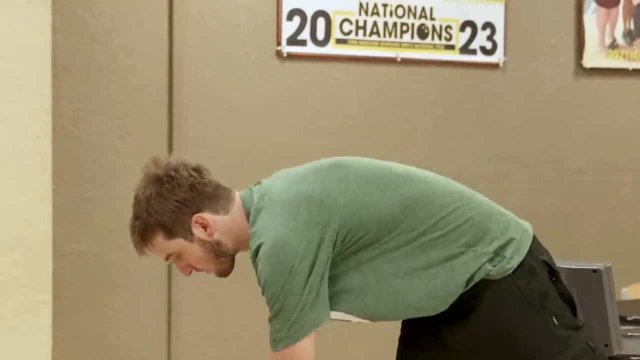 one for one, though obviously it has good pin carry duh. uh, i'm on my feet, two to the right, so i'm not sure if that's helping, hurting or somewhere in the middle, but uh, it seems to be like it's hooking a little more, not down lane, just. 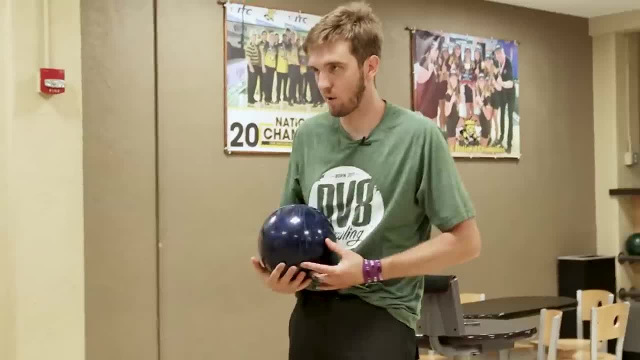 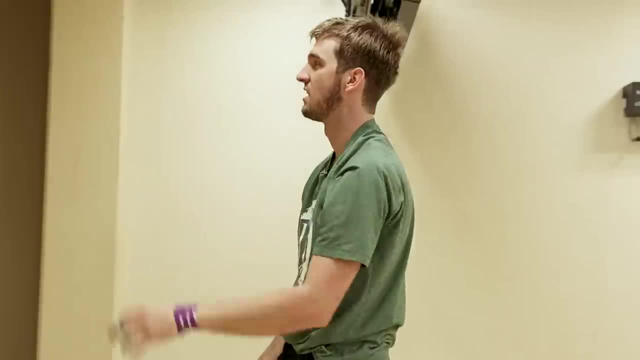 a little bit more, just a little bit more, and then i'm gonna go straight into the game. not a good shot, a little like more overall. also, i am two for two. i'm going to shoot 300.. that's a fact. i feel like it's hooking way less down lane. 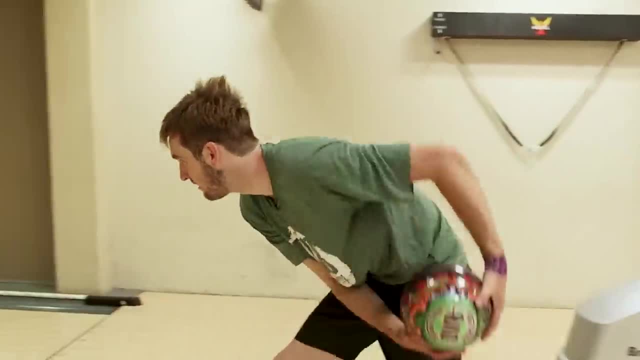 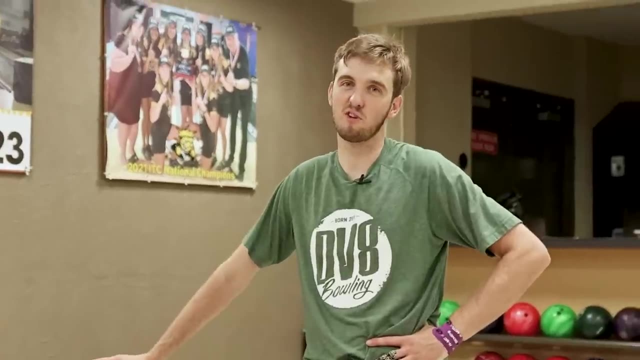 it's definitely hooking more, it's just hooking less down lane. that's disappointing. thought i made that. i think that's where it's harder than the bucket. i make buckets like it's my job. there's no way that's harder than the bucket i'm. i feel like i've made. 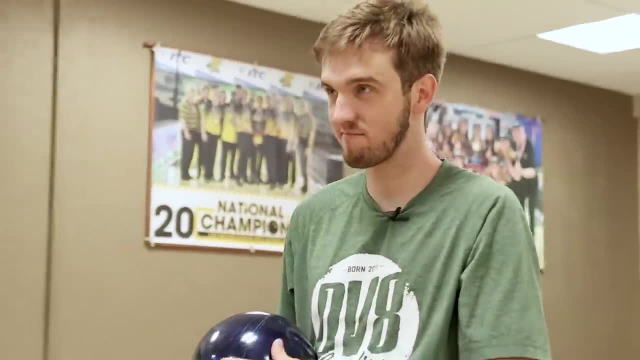 a million buckets and every time i make a million buckets it's harder than the bucket i'm. i feel like i've made a million buckets and every time i shoot that i like i find a way to get two. okay, it's hooking earlier, not as much down lane, i'm just gonna. 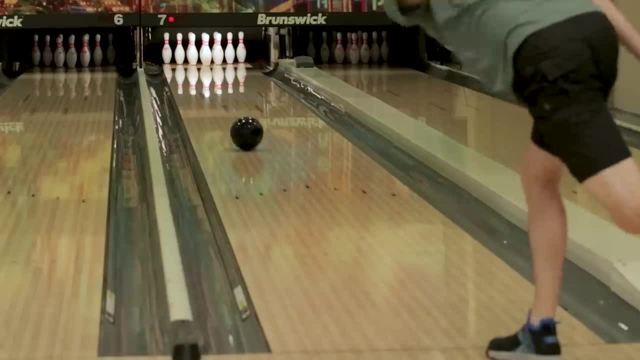 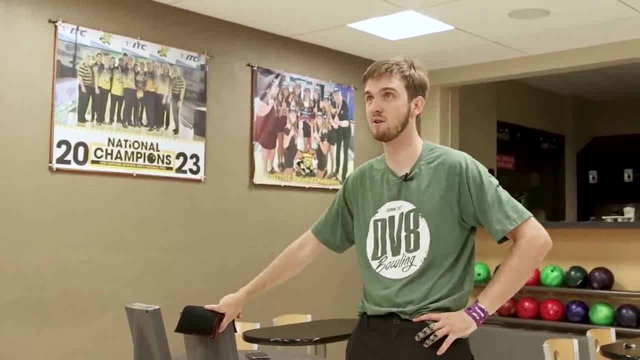 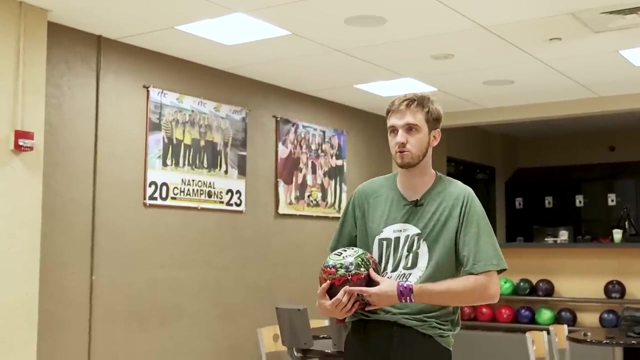 rotate it from the same spot. it's pretty responsive to what my hand does. i think i could hook this a lot if i wanted to like. i just rotated that a little more and it's booming down there, but the flare rings are much wider spread, which means it's essentially trying to hook more. 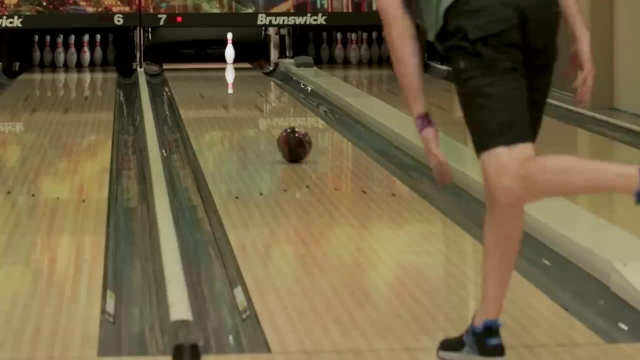 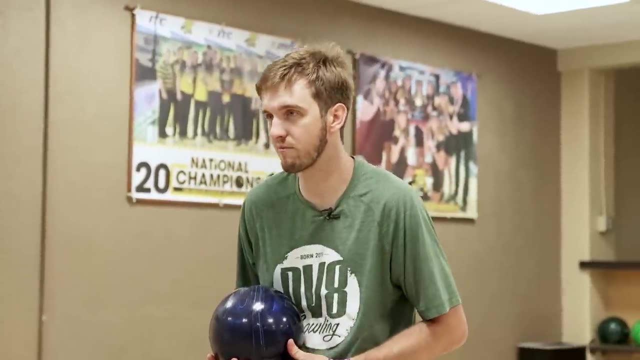 but the flare rings are much wider spread, which means it's essentially trying to hook more. i'm going to take a little step to the right here. obviously we're going on something not super easy, but i'm throwing it good enough where i can hit my target down lane every shot and 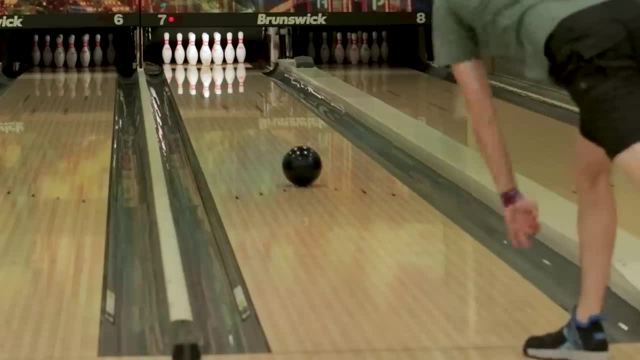 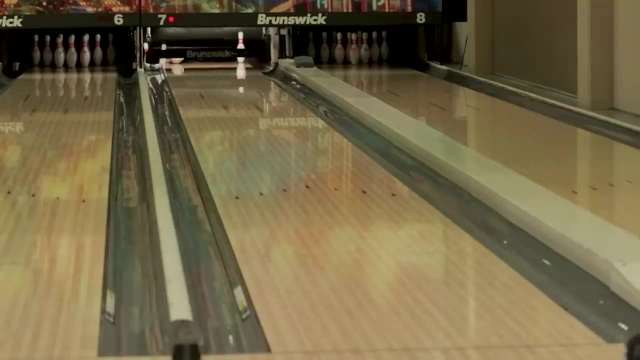 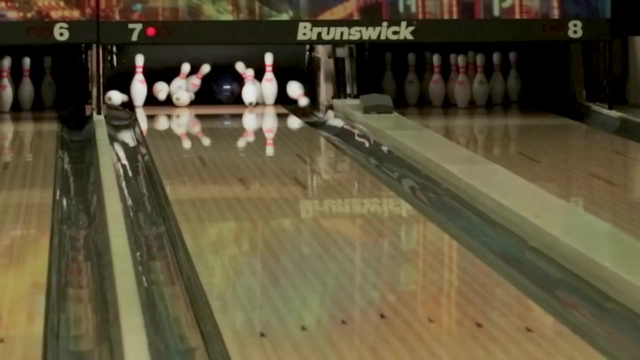 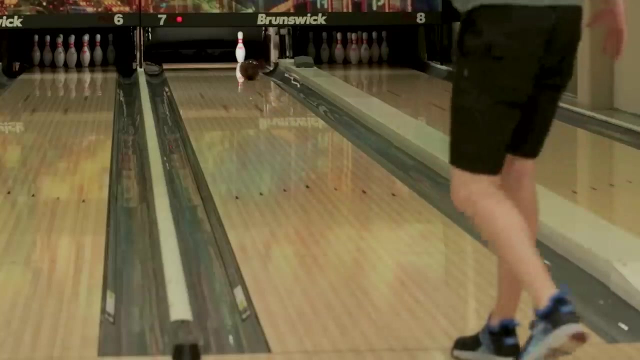 we'll see what the ball can do. the finish- like the ball freeze framing when it's going off the deck- has got to be like tackling the nine pin every time it has to be. if i want to shoot 200, i gotta probably triple or throw a couple doubles, so i'm just gonna keep. 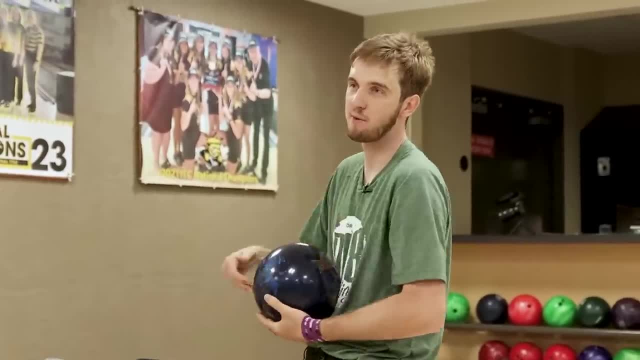 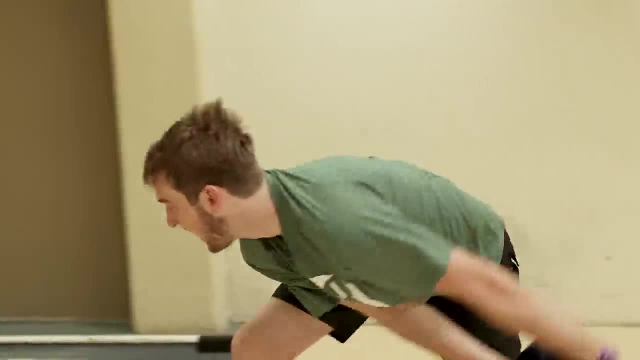 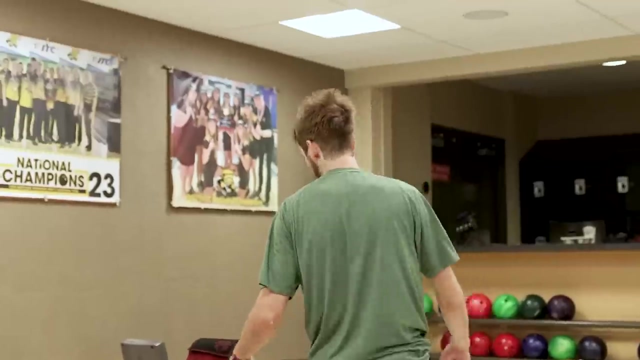 going right. why dial the hand down when you can just keep going right? well, i guess i was standing on 13 to start, so now i'm standing on 23, so i've moved a total of 10.. push, see the ten pin just late. yeah, that ball's definitely driving. yeah, i don't know if i'm going. 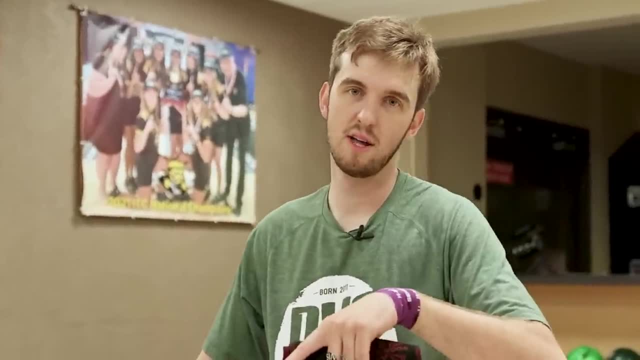 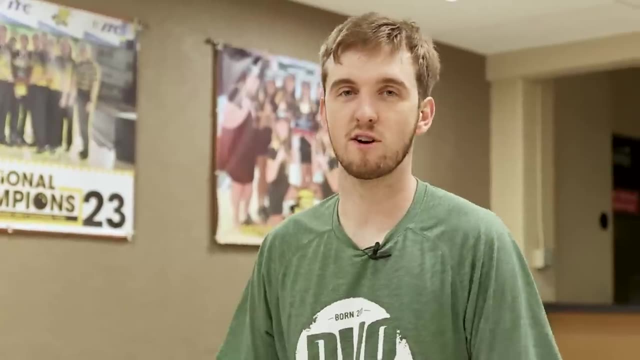 if it's the extra weight or the where the weight is in the ball that makes it do that, but i don't care. i'm gonna find a way to match this and throw it in pva competition because, according to all of you purple hammer haters, i'm a cheater. the flare rings were much, much closer together before that. 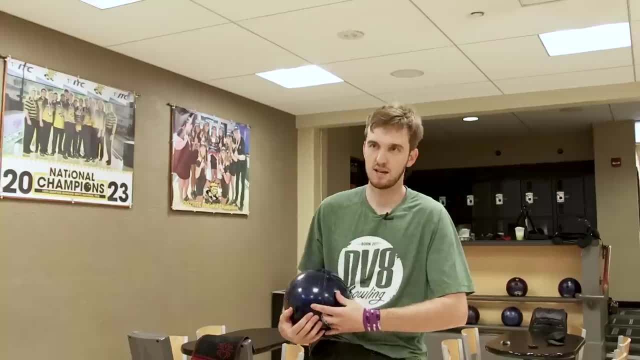 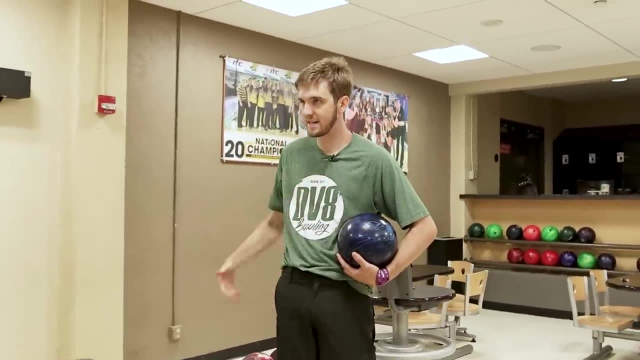 they were kind of probably was about half that size. yeah, usually balls that flare more try to hook earlier, which is what i think this ball is doing, but the cover stock is a little flippier, so it's still hooking a lot down lane, not just like a big ball would, where it would hook early and 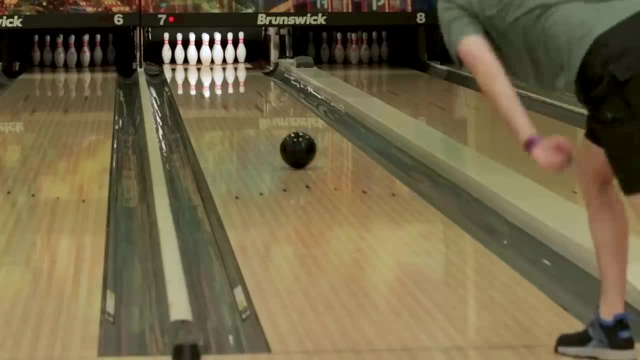 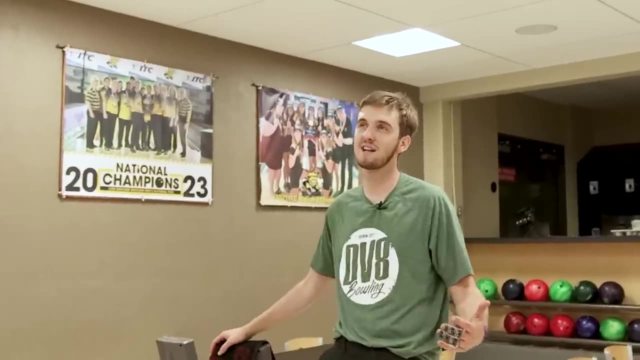 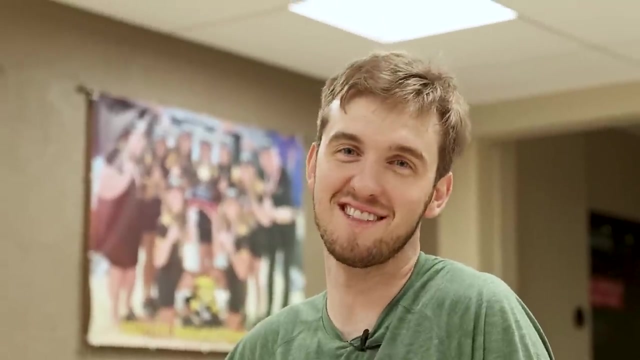 kind of make a very smooth motion. oh, that's such a bad shot. i'm a two-handed lefty. i put bolts in my ball. i'm going brooklyn. is there anything else i could do? like what can i what else? please let me know down below what more i can do to be cheating. 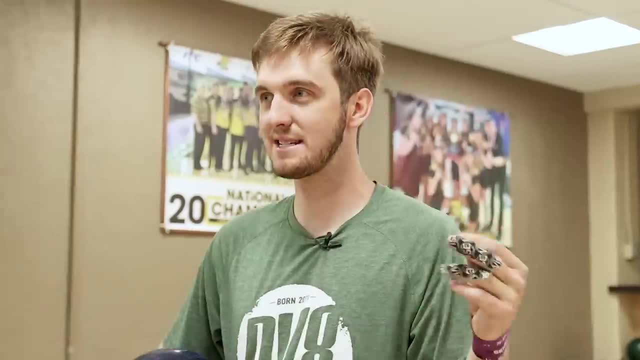 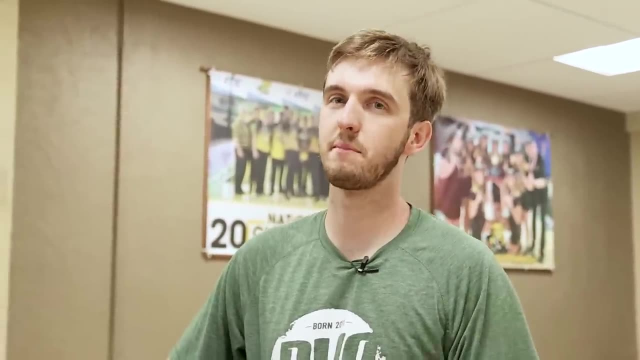 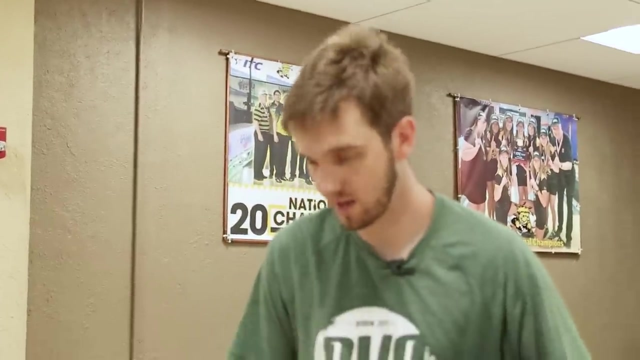 could i put a third hand on it. so matt did bring the inspiration of this video. have you guys ever seen anybody like that? you know for a fact- not like oh, he was cheating, but like you know for a fact- that either someone's done something like this or feel free to share your story down below. i'll try and read as many. 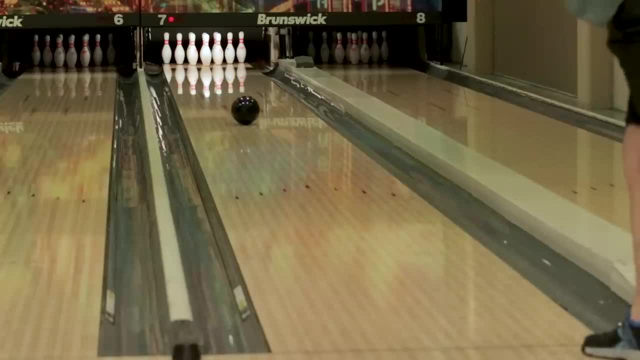 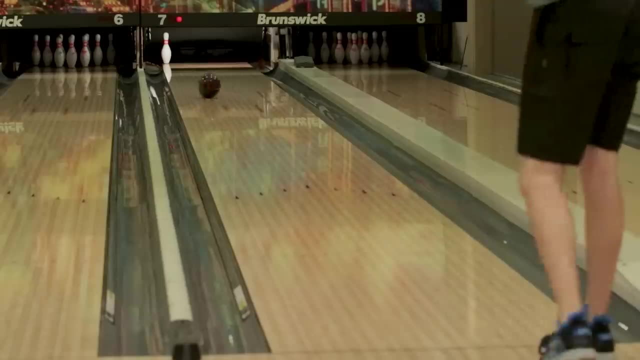 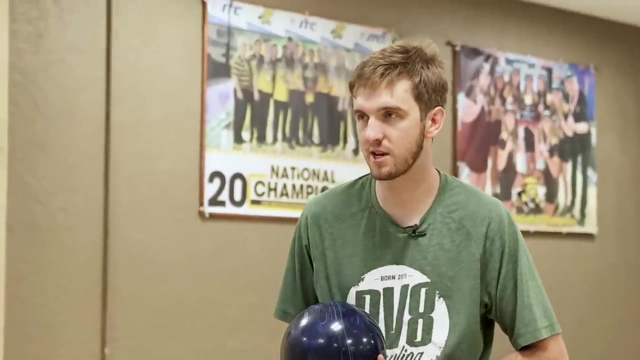 as possible. that's in brooklyn again. that's a ripoff. that's what that is. i'm allergic to missing spares. i'm gonna do a little bit of a. i'm gonna go another three to the right, so i'll be 18 further right of where i was standing earlier. 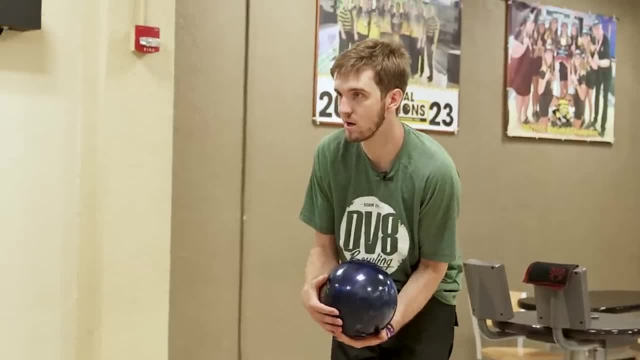 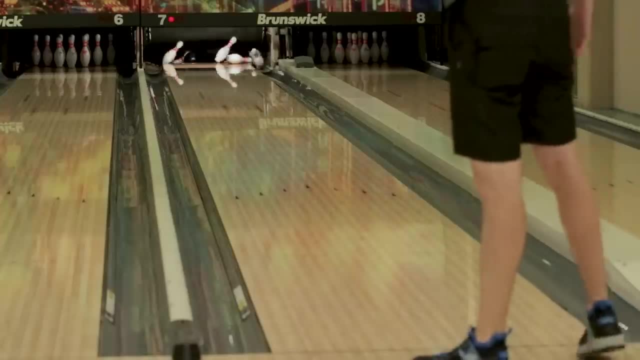 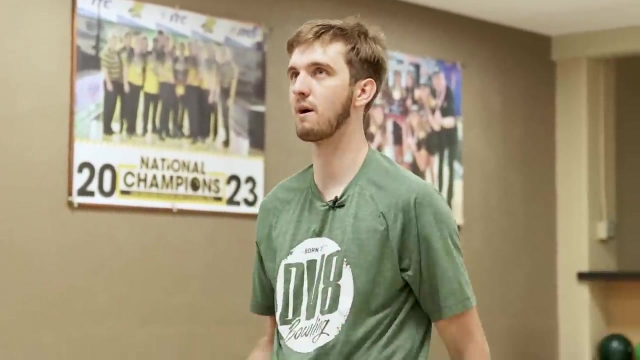 obviously rotating it a decent amount more, but it keeps hooking, so i'm gonna keep my eyes a little closer to me. that is the spot where i feel like i'm lined up at. maybe i would go a little further left and like play a little straighter. but for right now, just to show you guys how much this. 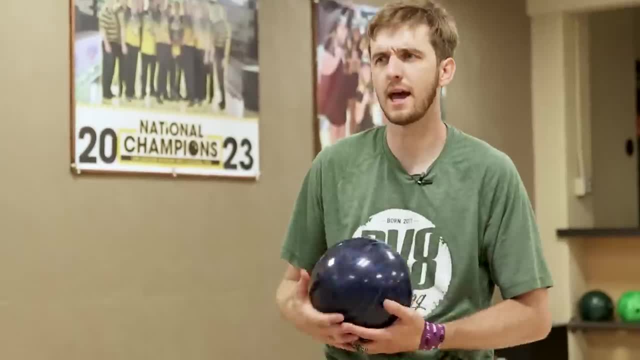 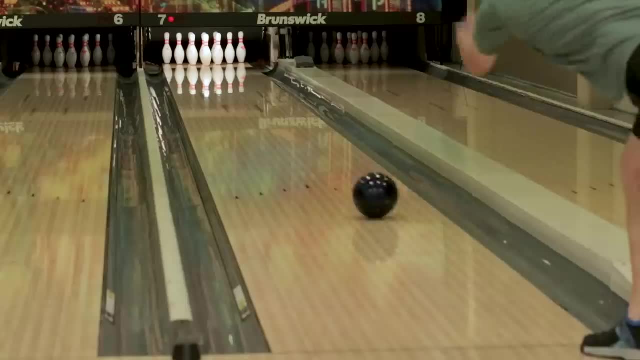 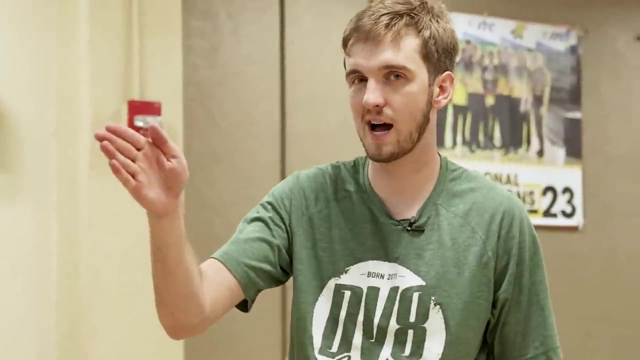 ball can hook, is it? is it hooking more than what you expected? yeah, i thought it would hook a little bit, but i think it would make that much of a difference and it's clearly making a massive difference. and, like every time i get like that, that was actually like decently online, but just a little. 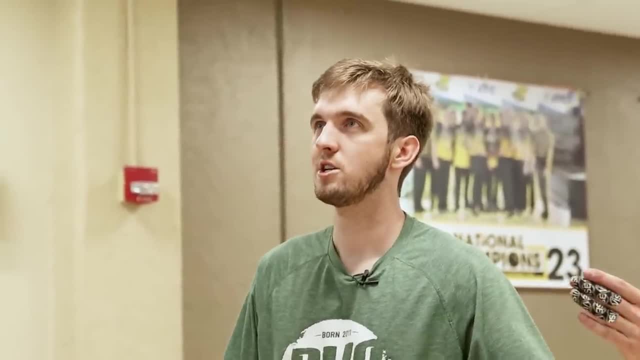 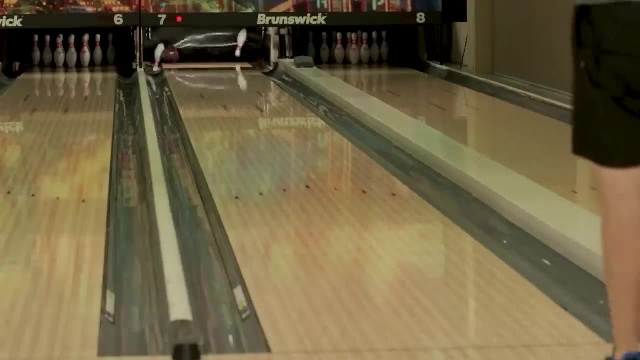 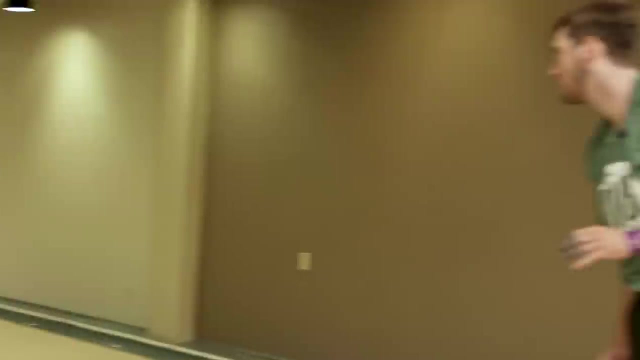 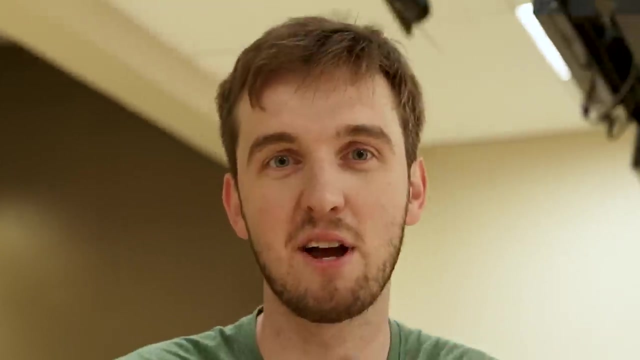 too much rotation. i got around it a little early and it like knifes down lane. that's a big time spare, spare for 200.. as i said, i mean, i am allergic to missing spirit. that's brooklyn again, it's not about how you start, it's about how you finish. thank you guys for watching. that was my. 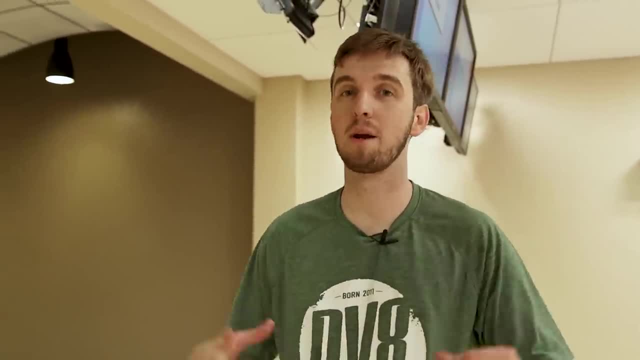 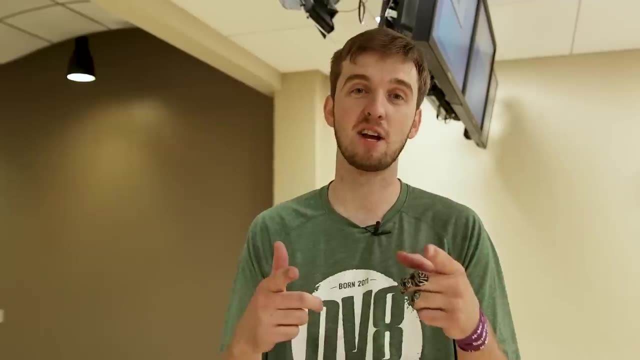 super illegal bowling ball. you watchers put some bolts in it and create a massive amount of side weight. let us know if you've seen anyone cheat or do something similar to this down below in the comments, and i'll catch you guys on the next one, don't forget. if you guys want to see a little more,